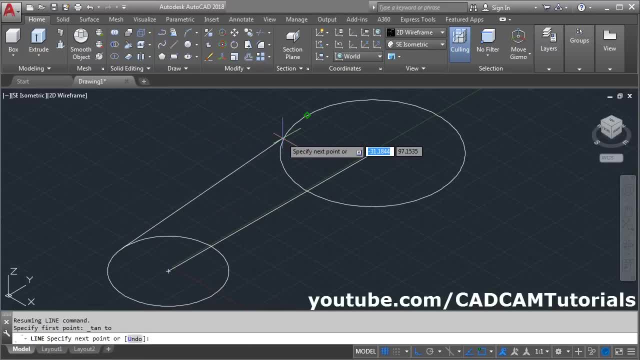 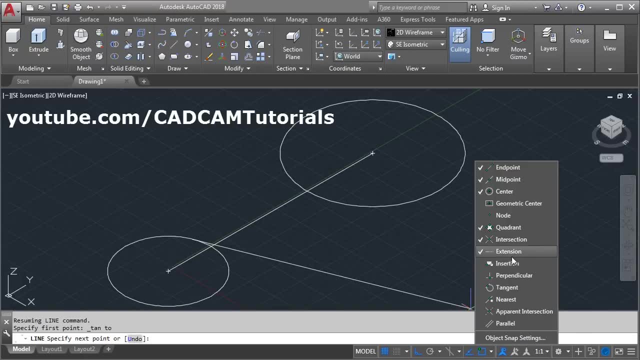 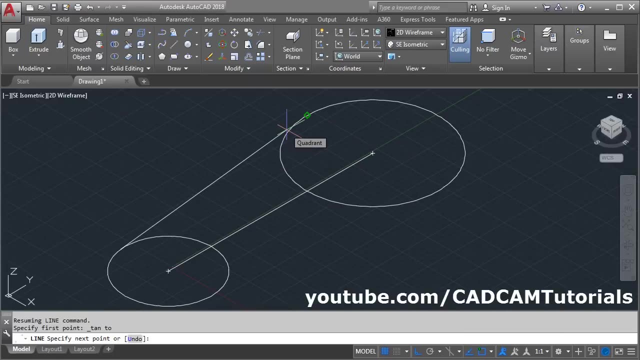 It is the first method method. Second method is you can make it on from here: Click on the circle. That is the first method. Second method is you can make it on première here: click on the arrow, then select tangent, click outside. now here, even though I have said tangent it. 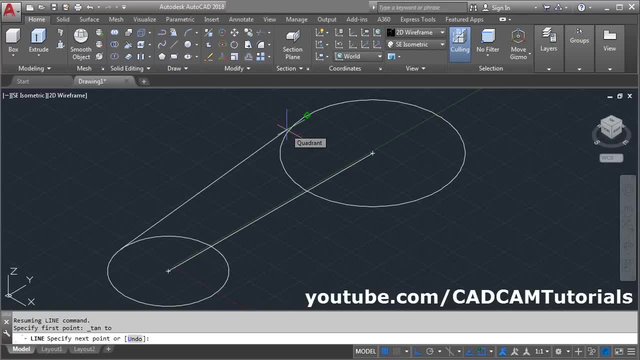 is showing me the quadrant. that means I will have to make this quadrant off so that it will show tangent. click again on this arrow and make this quadrant off and make the center also off. then click on the circle, enter, then again enter to repeat the line command again click here and click here and press enter. then it. 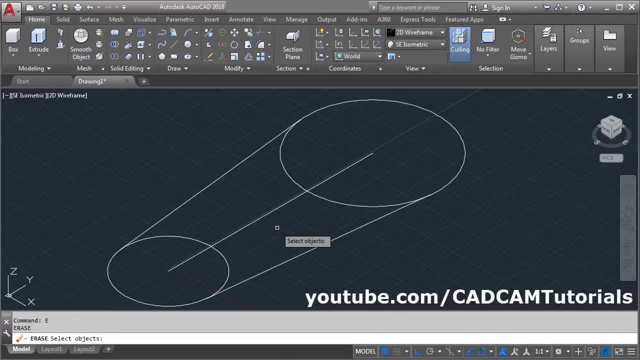 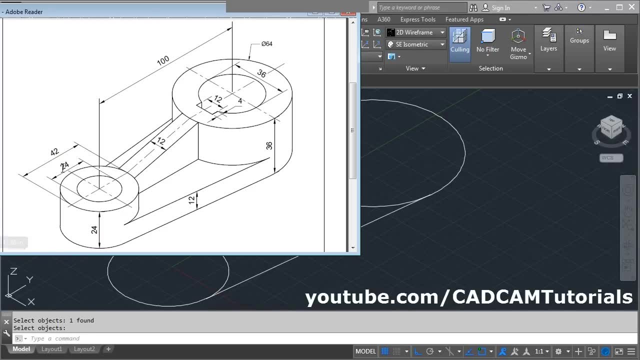 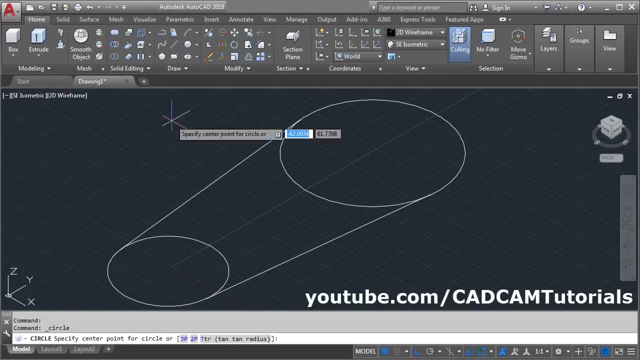 is the internal line. give E enter, select the line enter. then two internal circles are there of 24 diameter and 36 diameter diameter. again take the center diameter command. give the center point. now center point is turn off again. we can make it on from here. make center on, click outside. 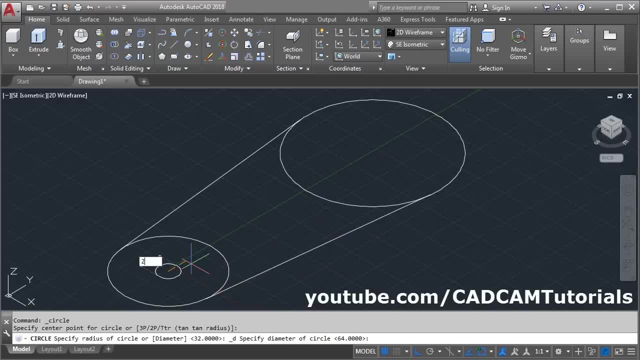 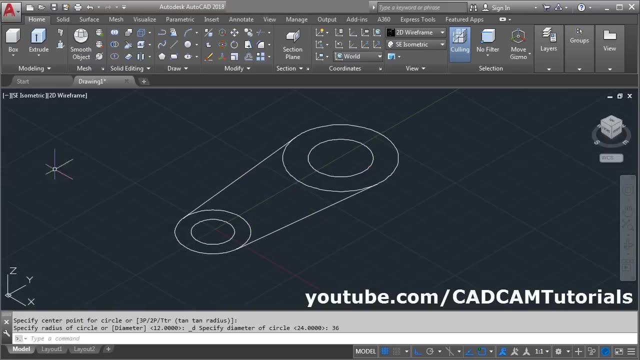 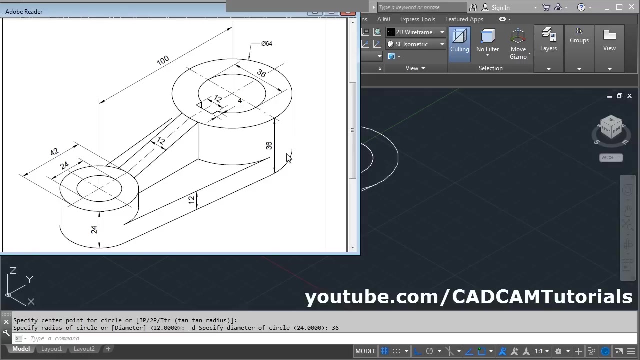 give the center point. diameter is 24. enter I can give the center diameter. I can give the center point. give the diameter of 36. enter this internal portion. we will need the thickness of 12 for this. here is the 12 thickness for this internal portion and this portion height is 24 and this portions height is: 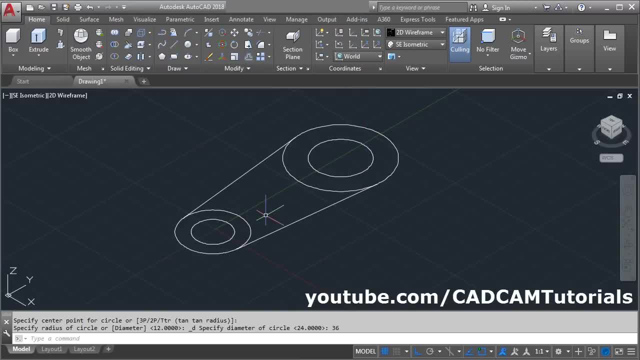 36. to convert this object into 3d, click on press full. give some time for it to get started. then take your cursor inside the shape, click there, give the direction. I want to go above and give the thickness of 12. enter now. press pull is still running. we can. 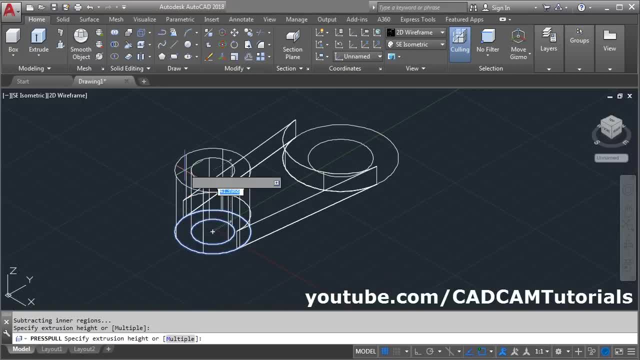 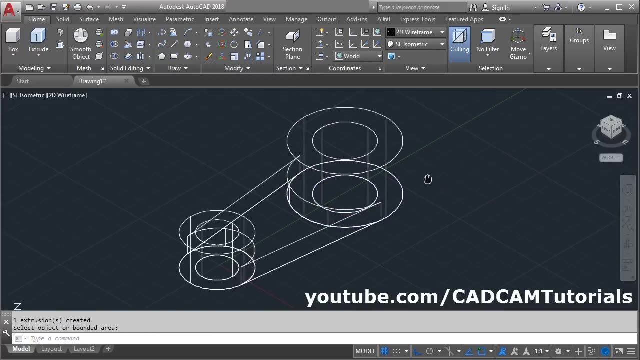 again. go inside these two circles. click there, give the direction, give the height of 24, enter. then take your cursor between these two circles. click there, give the direction, give the height of 36, then enter. to stop the press pull command. pan it for 3d. look, click here on 2d wireframe. 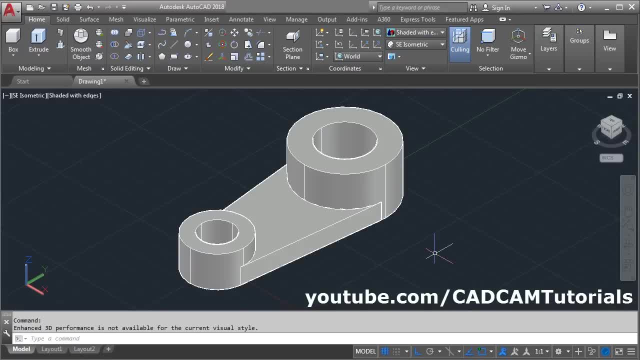 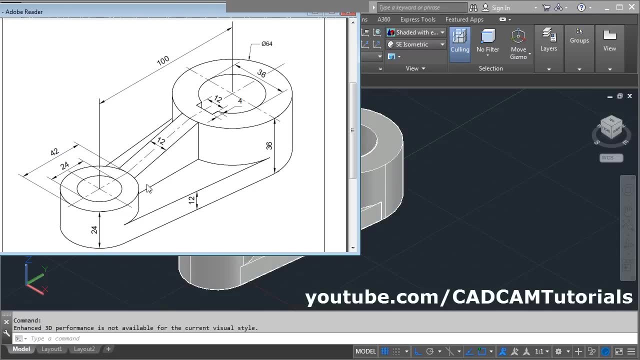 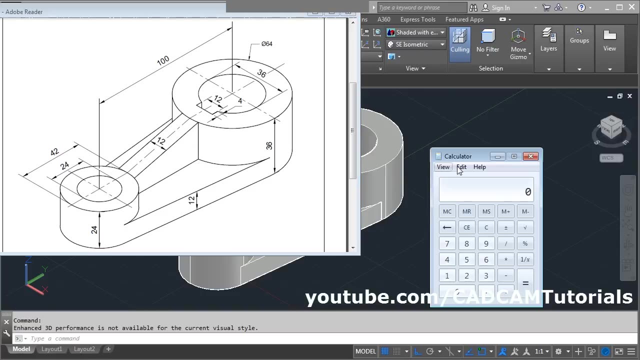 and select this. shaded with edge is so it will be shown in shaded mode. then next will be internal drip of 12 thickness. at first we will have to work out the length of this rib. for that we will do some calculations. we will take calculator now. here. the length will be 100 minus radius of this circle, minus radius of 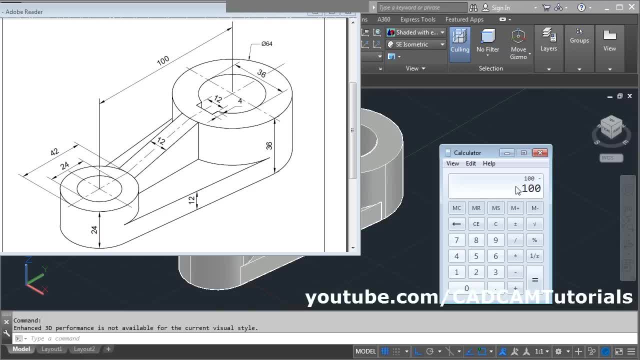 this circle. so we will take it 100 minus it will be: pop up: 42 is 21 minus hop up, 64 is 32. that means 47. the length of this rib is 47, then here height will be 36 minus this trail, that is 24. and here it will be 24 minus this. 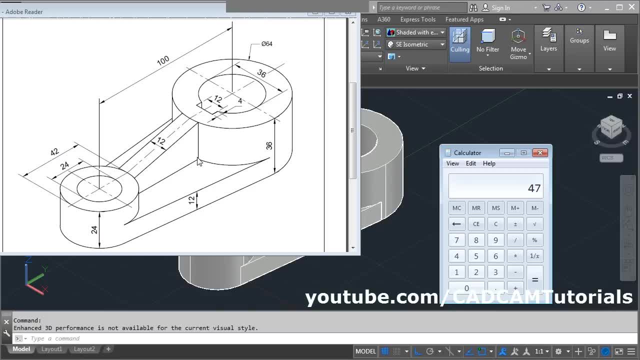 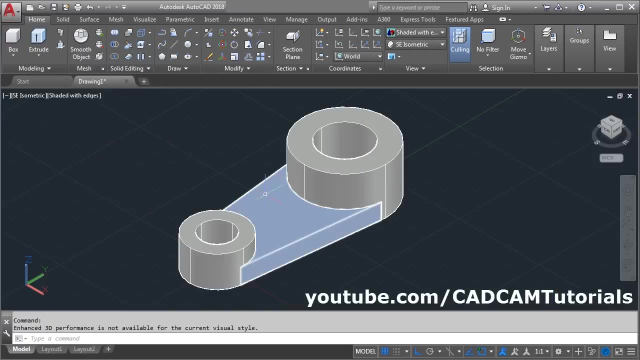 trail. that is 12. that means 12, 47 and 24. now this rib is vertical. to create this rib we will have to change the plane. we will have to create this shape and press, pull it in horizontal direction. for that we will have to use right plane. that means we will have to make this XY vertical to. 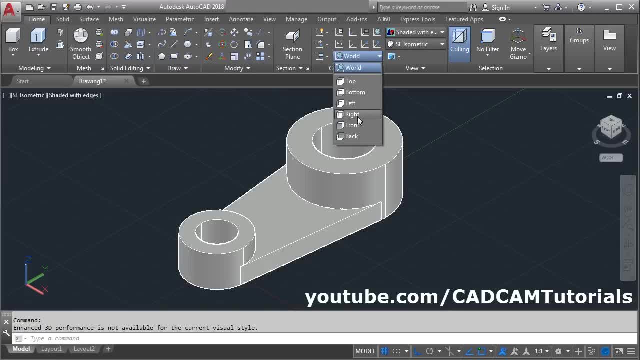 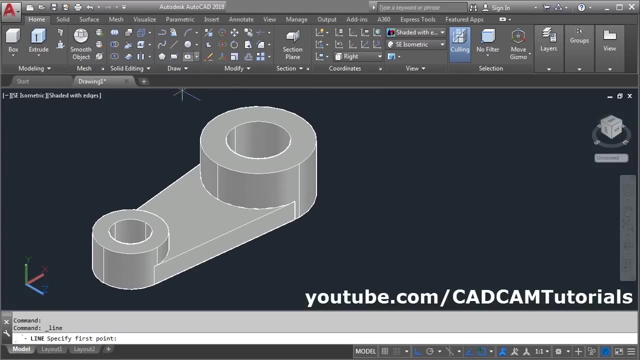 change the plane. select here and click on this. right now, XY has become vertical, as we require. if you don't want this grid, you can make it off by clicking on this button here and take the line command. give the first point, take your cursor down. give the height of 12: enter, take your cursor. 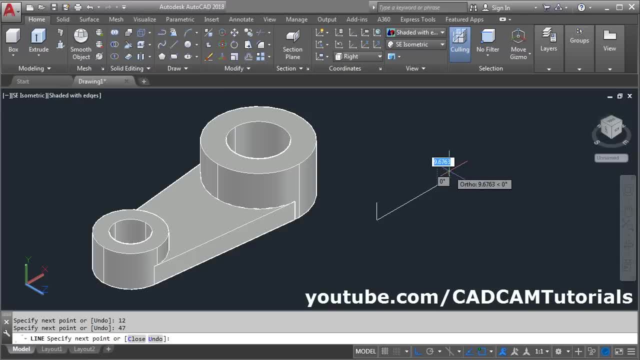 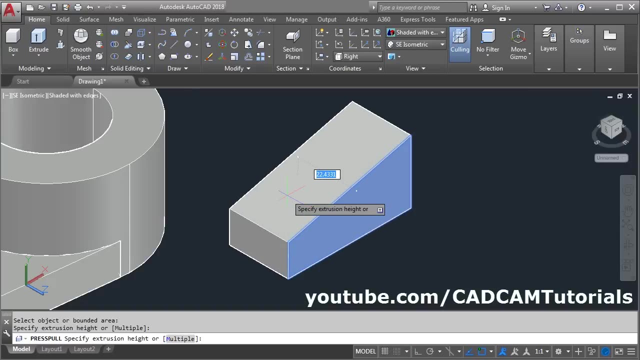 on this side. give the length of 47, enter. take the cursor up. give the height of 24, enter. then connect back to this start point and enter, zoom it and press, pull it, press full click inside. give the direction, give the thickness of 12 and 2, then escape and we will have to do. 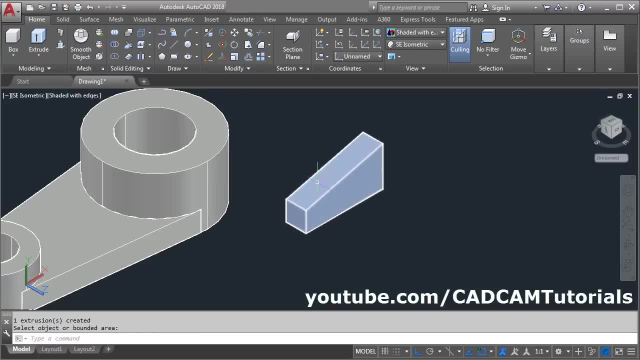 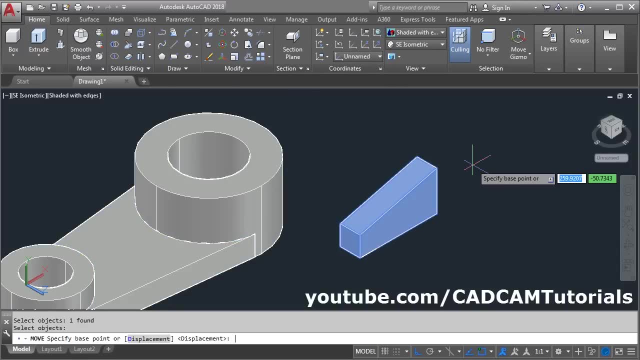 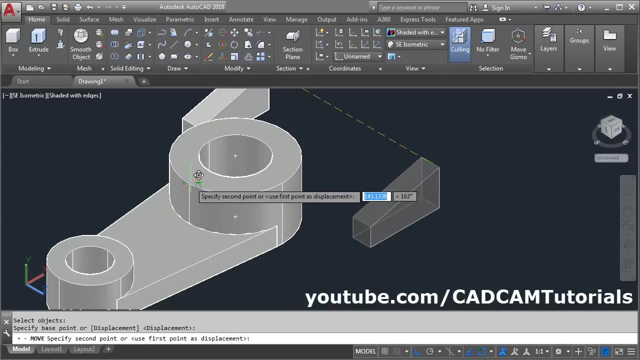 ones that are behind and two that are behind the hip joint eternt. so now we gone and see how to make our size of theทำ. move it and place it here. select, move. select the object, enter. we will match the midpoint of this line with the quadrant of this circle. now it is not showing the quadrant, we can shift right click. 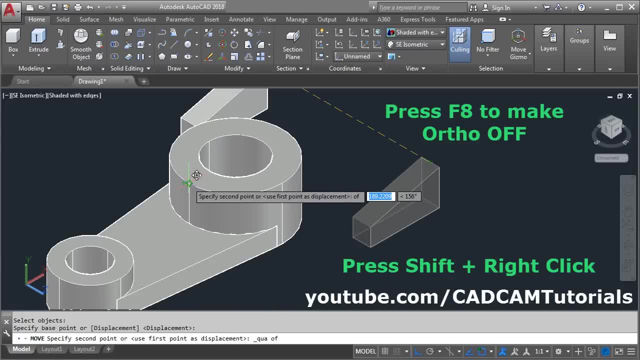 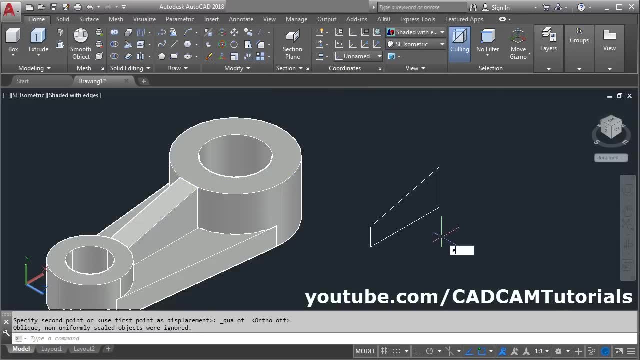 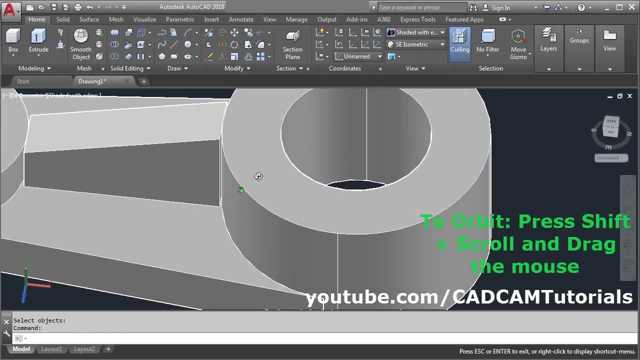 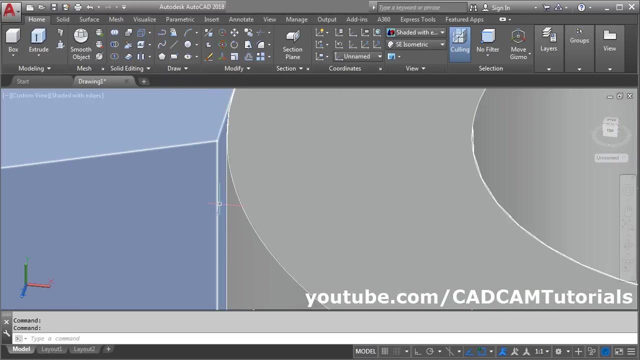 and select quadrant and place there we can make ortho. press f8 and click erase these lines. e, enter, select all the object, enter. now this rib is placed here, but if we orbit it to orbit, press shift, scroll and move the mouse, zoom here. now. here we can see that there is a gap. actually we don't need this. 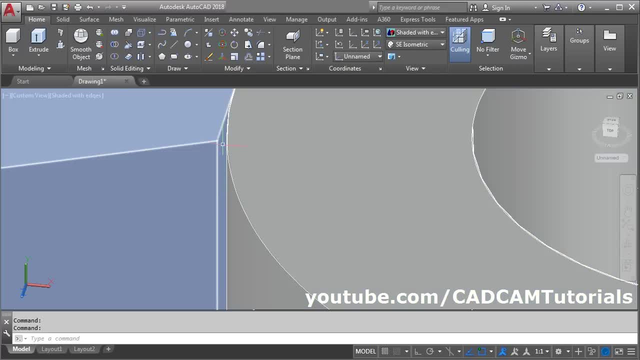 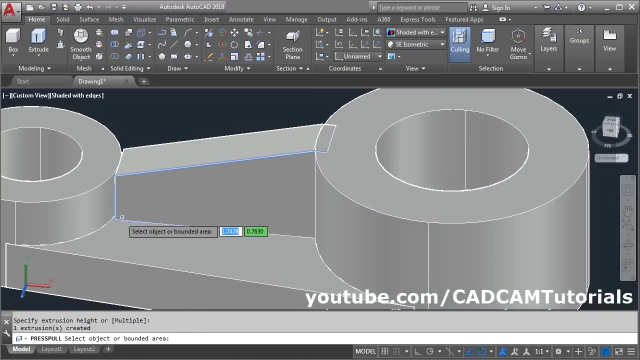 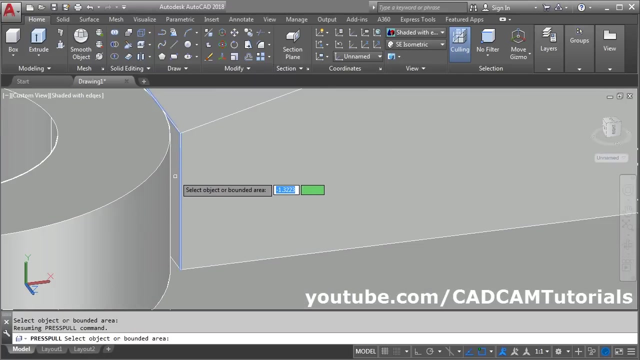 gap. to fill this gap we will again have to press pull this vertical portion. for that again, click on, press pull, select this internal surface. take the cursor inside this vertical cylinder and click there. same way, if you orbit here, press shift, scroll and drag the mouse and zoom here. here is also gap, is there? click on this surface, take your cursor inside and click. 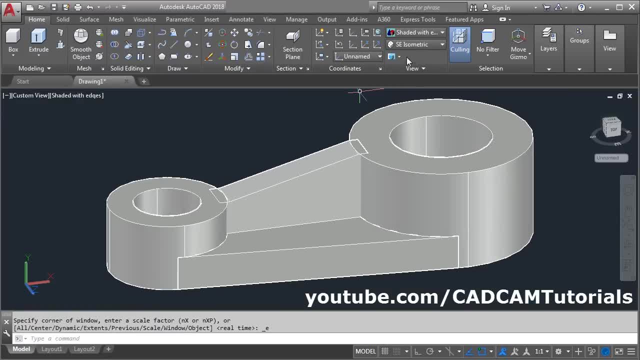 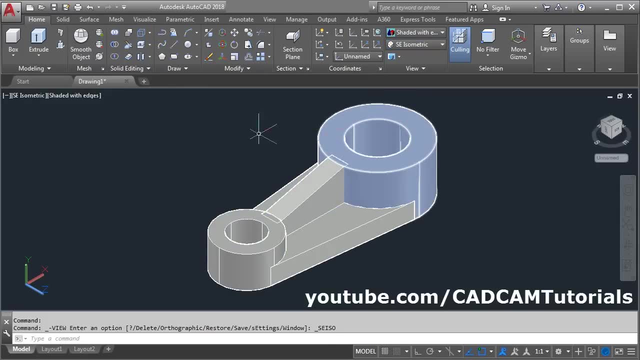 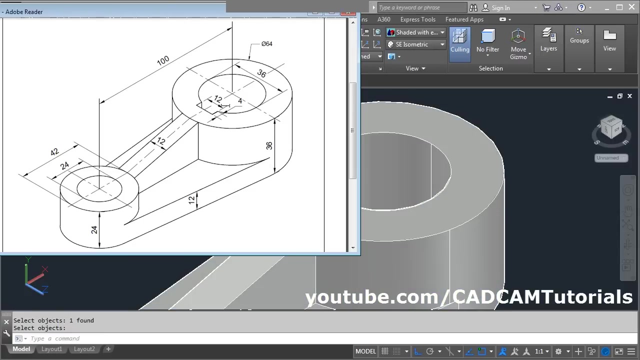 enter, zoom, extend and from here we can click on ac isometric. now these objects are separate. to combine all these objects, use the union command. here is solid union, click on it and select all the object and enter. the next is this keyway of 12 by 4. now this keyway needs to. 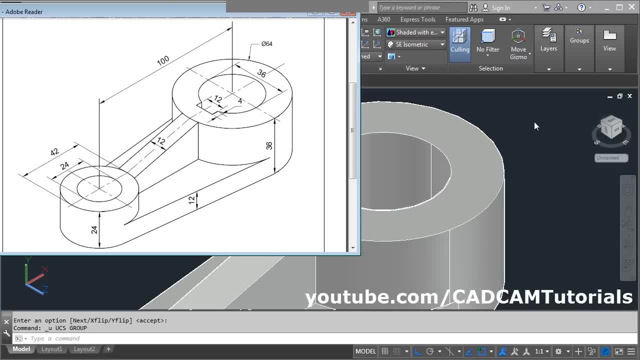 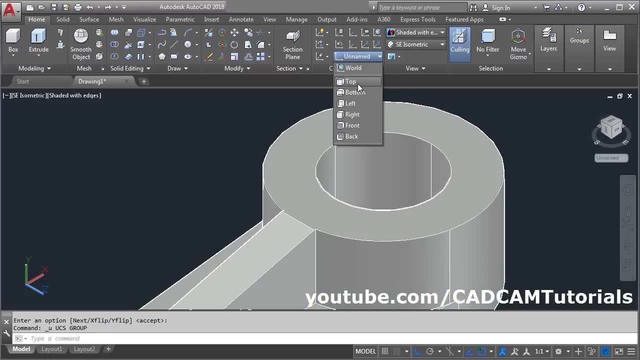 be made on this surface. for that we will have to change the plane. now this surface will be a top surface. for that, click here and select top, so our x, y will become horizontal, that is parallel to this surface. then take the line command. we will create one line from the center of the surface. 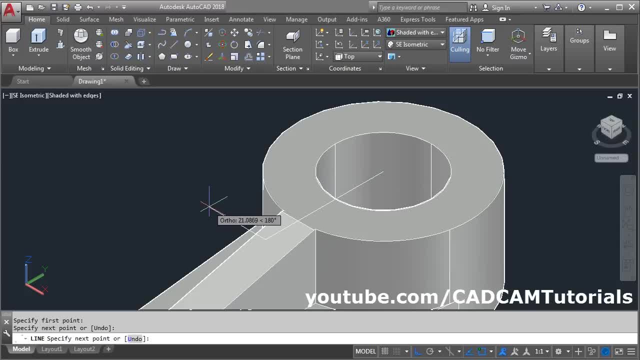 center of this circle. take it outside and click and enter. then we will offset it. click on offset. give the gap of 6. select this line. take your cursor on this side. click there again. click on this line. take your cursor on this side and click there and enter. 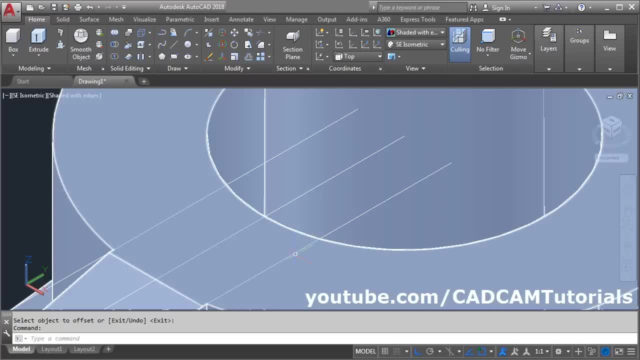 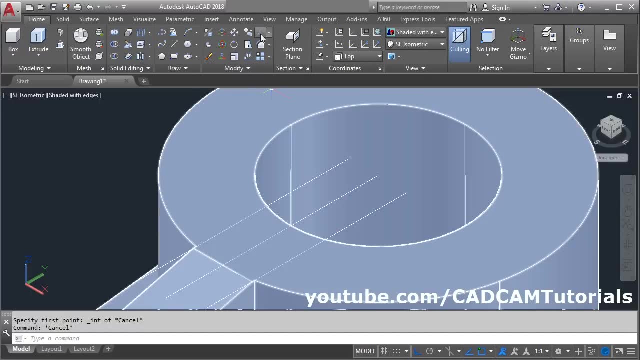 now we will need the length of 4 from this intersection point. to get this point we will trim the unwanted object. give the trim command, click on trim, then press enter and click on the object to be removed. enter now we will need the length of 4 here. 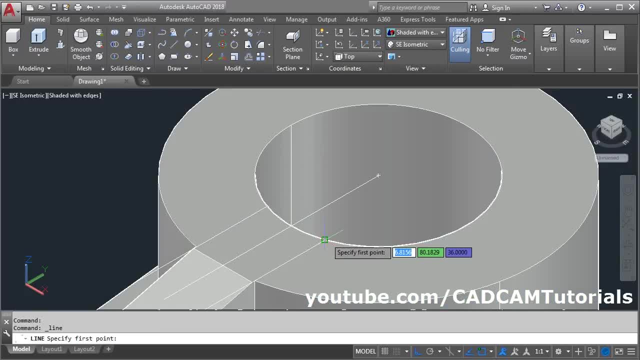 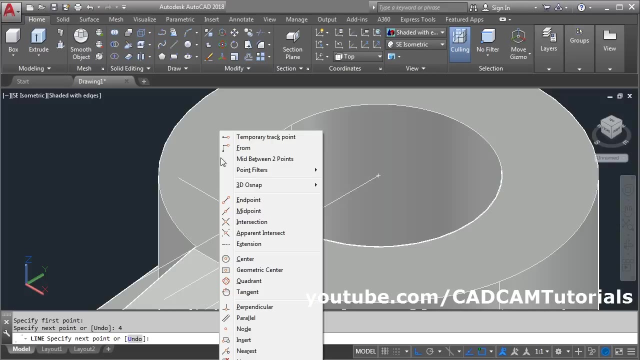 take the line command, take this end point, give the direction on this side and give the length of 4, enter. then take your cursor on this side. now we want this line to be perpendicular to the center point, so we will use this line and we will make it perpendicular to this line. press shift and right.